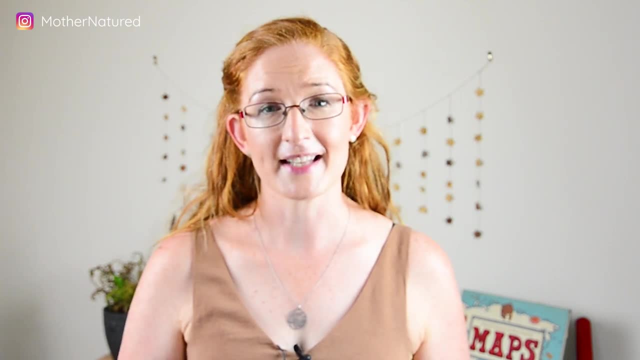 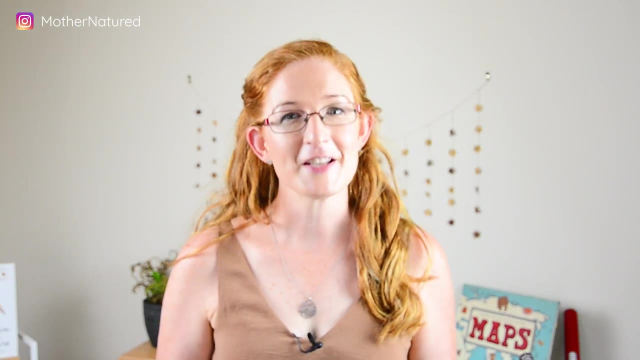 let you know that we tested different glues for nature crafting recently and there's a glue that works really well and you probably have all the materials in your home, so I'll link to that in the description below. The second tip is to bring nature sounds into your home. If you can't bring 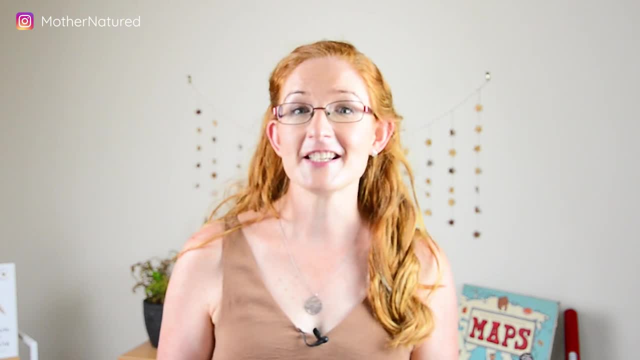 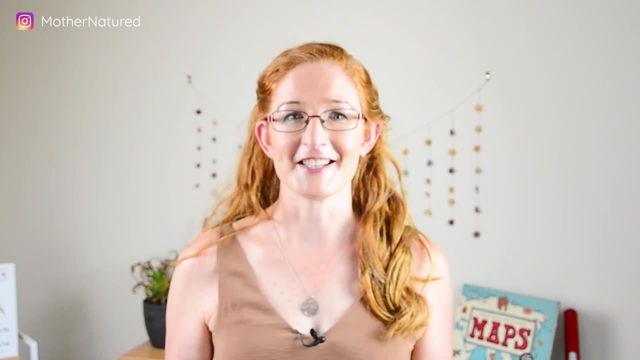 nature in the house because you're just not allowed out. then bring nature sounds in. Go to YouTube, Spotify or any music app that will allow you to search and download some of the nature sounds. Have it on as background music and I can guarantee you that it will add some soothing. 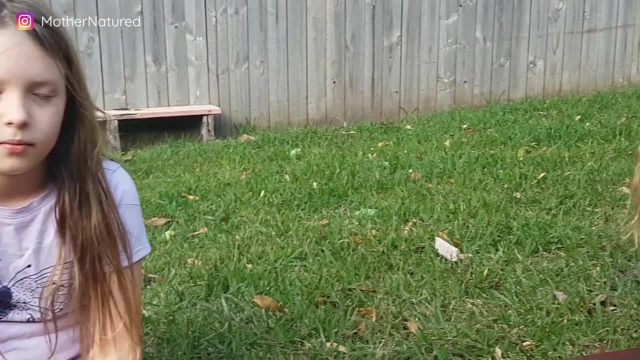 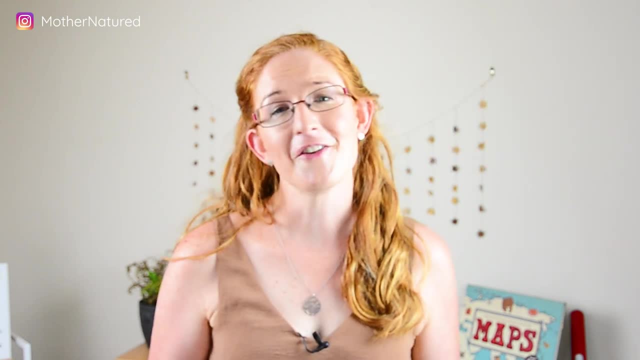 ambience to your home. You may even like to try meditation. I talk about the meditation app that we use in this video. It's all about our self-isolation. Try closing your eyes and listening to the sounds, just to enjoy it, and later see if you can get your. 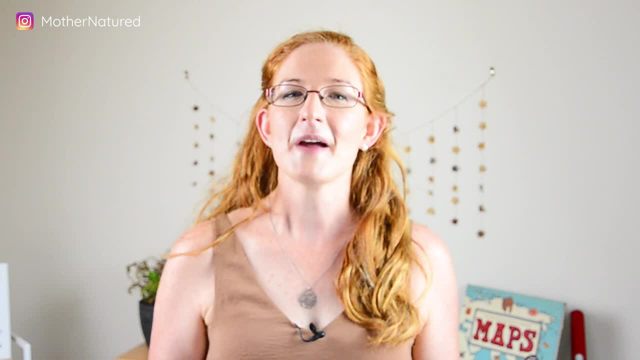 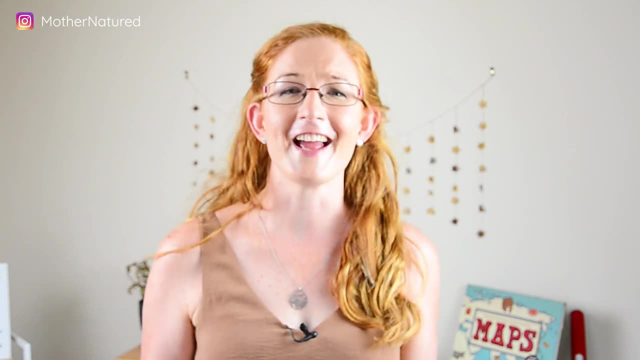 child to count how many bird songs he or she can hear. Make sure you change your tunes up too. For one week you could listen to the rainforest sounds, and then next week it could be the ocean, and then maybe a wet landfill with frogs and crickets. If you focus hard enough, your imagination will take. 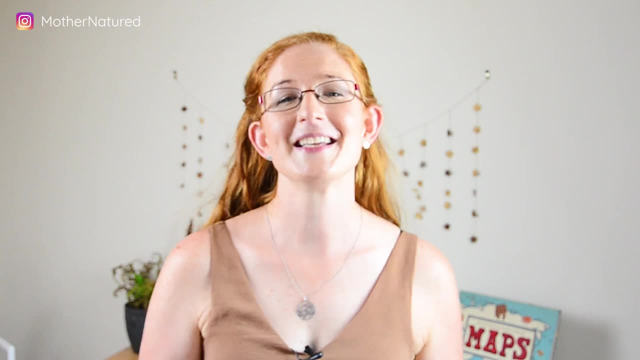 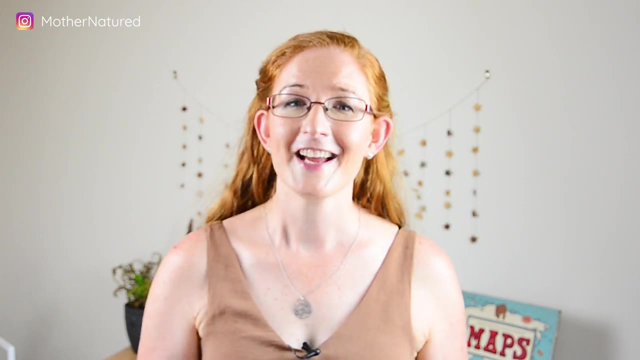 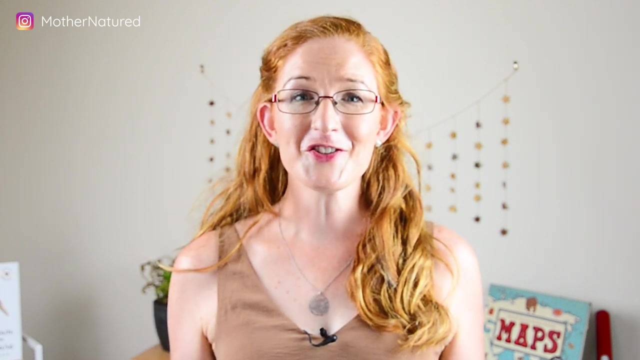 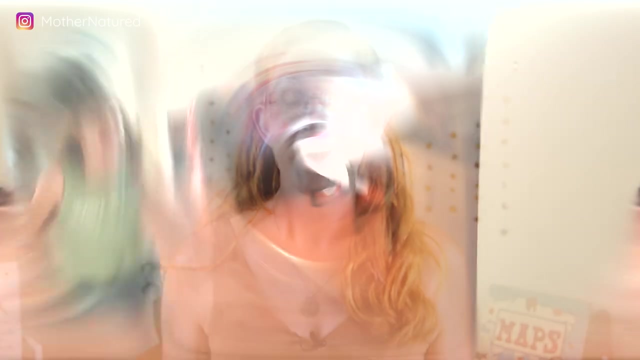 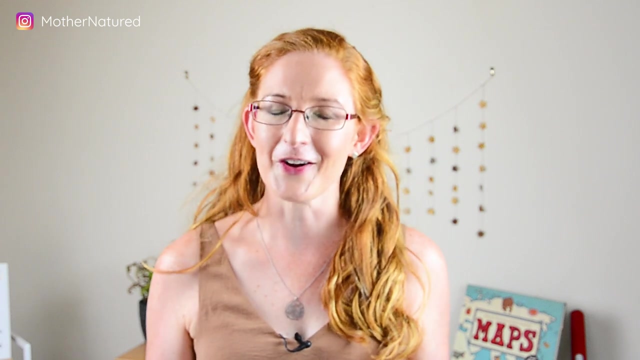 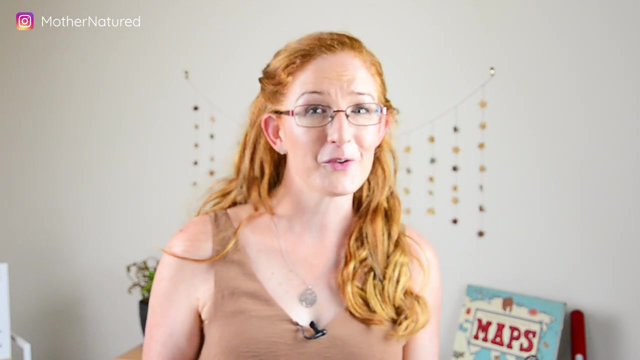 you right there. If you're finding these tips beneficial, please give this video a like. It means the world to me because it really helps spread the word about nature. I'll see you in the next one. If you can't find stray critters around your home, then set something up. Put around all your kids. 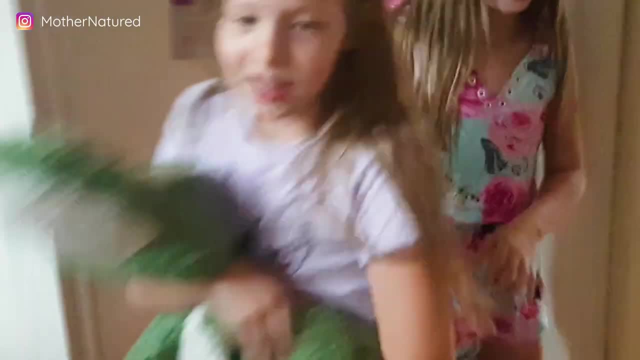 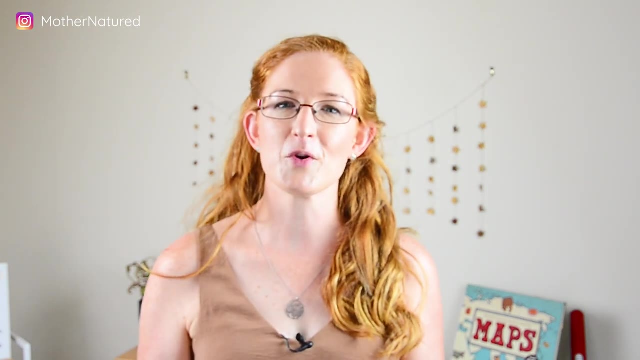 wildlife stuffed toys and get them to go on a wildlife hunt and see how many they can find. My next tip is books. Go and raid your child's bookshelves and find every book you have with nature in it. Or if you don't have some, you can order a couple on Amazon. I'm just going to show. 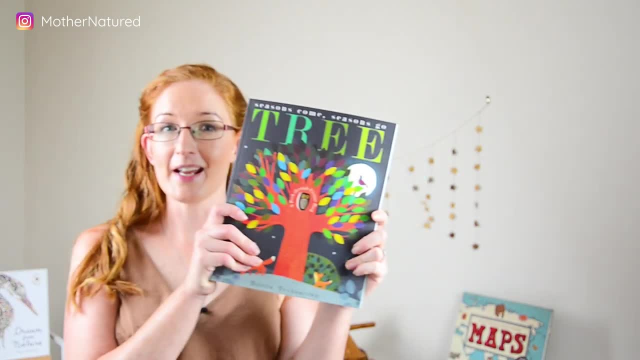 you a few of our favorites. For little ones, I would suggest Tree. It's such a beautiful book. It's by Britta. I'm not even going to try it. I'm going to give it a try. I'm going to give it a try. 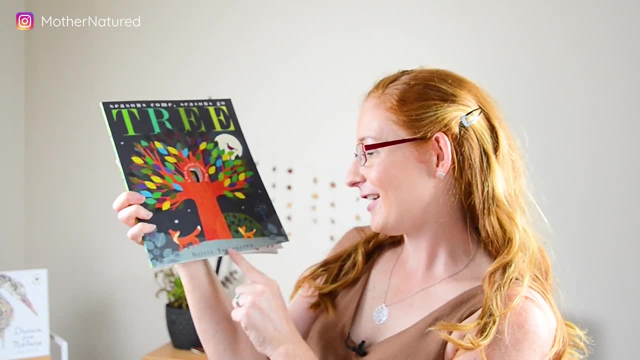 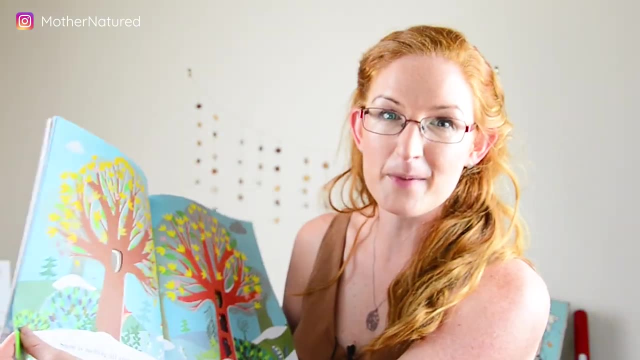 Her last name. I'm going to try it: Tech and Trap. Tech and Trap. It's such a beautiful book. It takes your children through the seasons and they have to spot. they spot different animals throughout the seasons and it just shows the cycle of nature. It's just a beautiful, beautiful book. 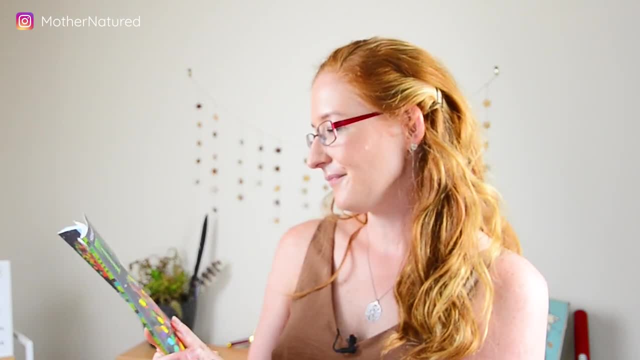 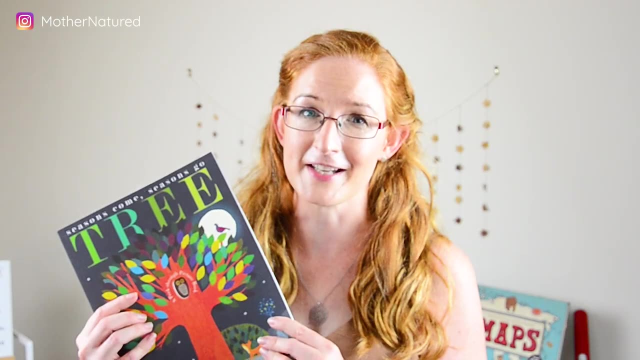 I bought this a while ago and the girls were a little bit big for it, but I'm actually keeping it because it's just so pretty and hopefully, when my nieces and nephews get to come back over again, I can read it to them. Another book we really love is: 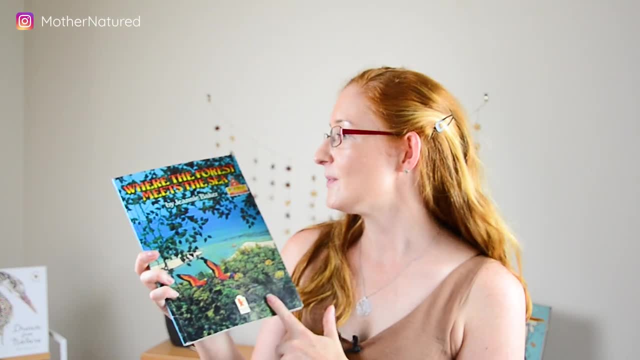 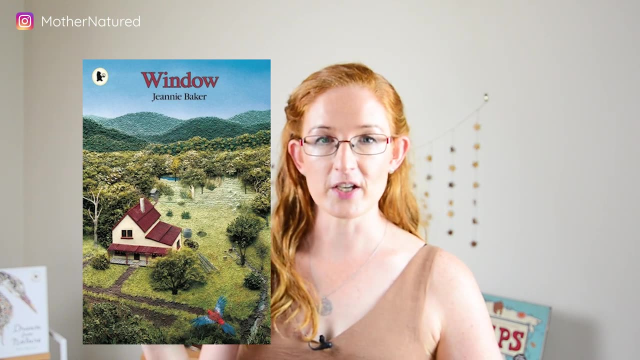 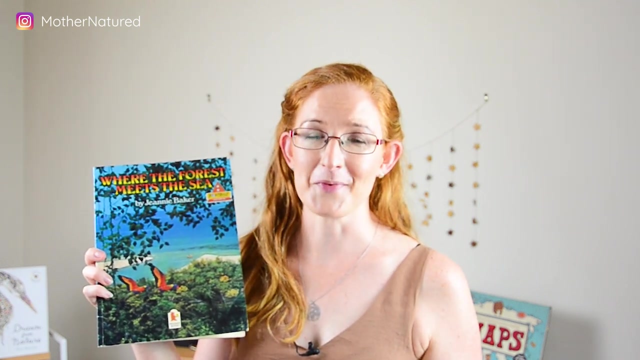 Where the Frogs Go. The Forest Meets the Seed by Jeannie Baker. She has this book and she also has another book called Windows that we usually borrow from the library, and Windows shows the progression of change over time by looking out the window, which is really, really good for the current situation we're in. 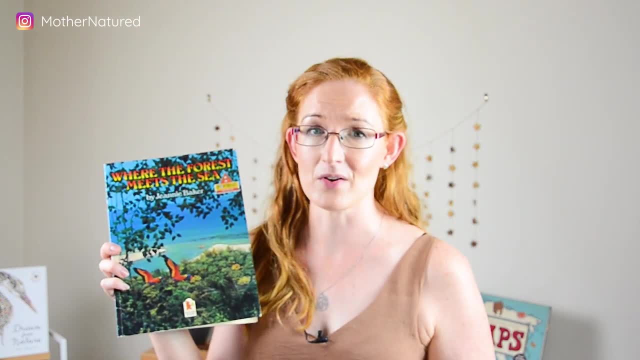 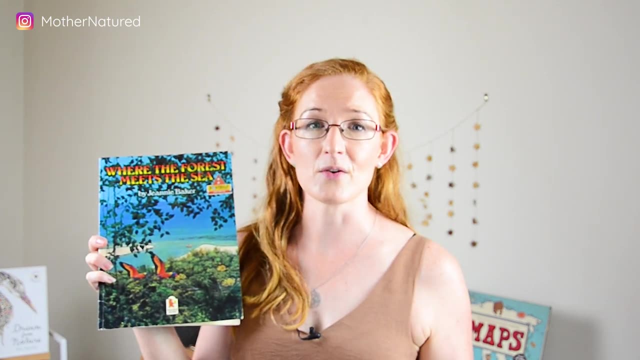 because many children are stuck inside and so they'll be looking out the windows a lot more and maybe they can start to notice little subtle changes that are happening. So that book is really beautiful. It also shares a really good message about the change over time and what's happening to the environment. and the same as this one, This one is a. 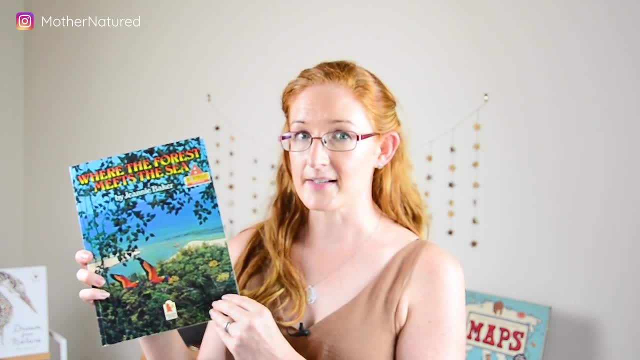 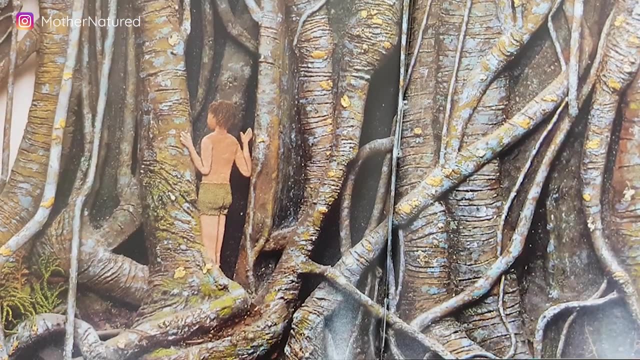 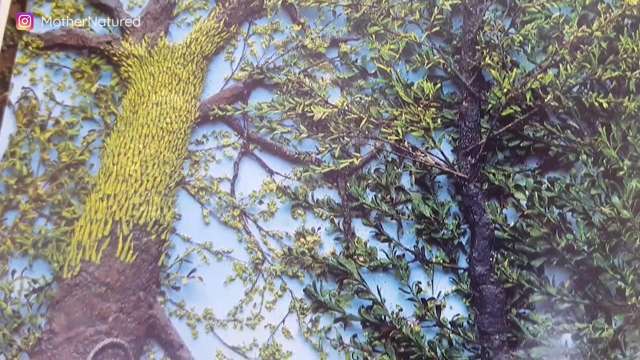 real, slightly environmental theme to it as well, where a child and his father go and find a secluded spot in the rainforest and near the beach. and you know, they think about the future and they think about the past in form of place. So this is a really lovely book and the images are just stunning. 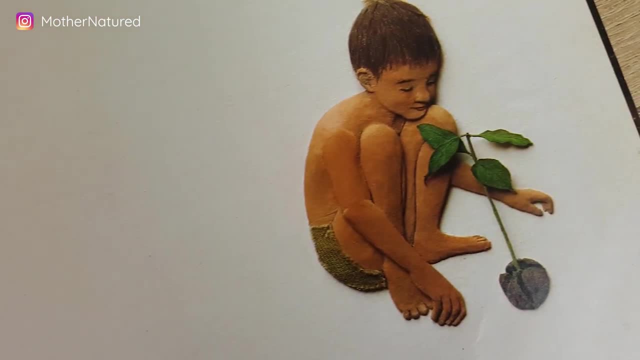 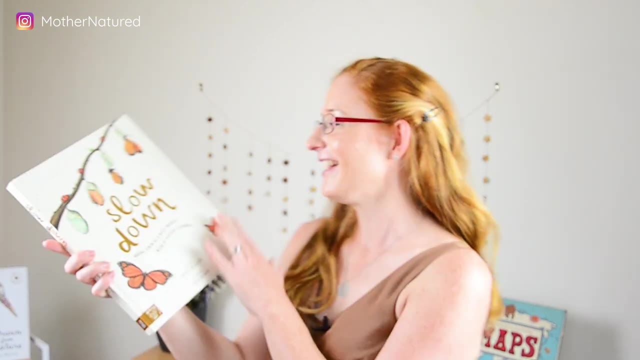 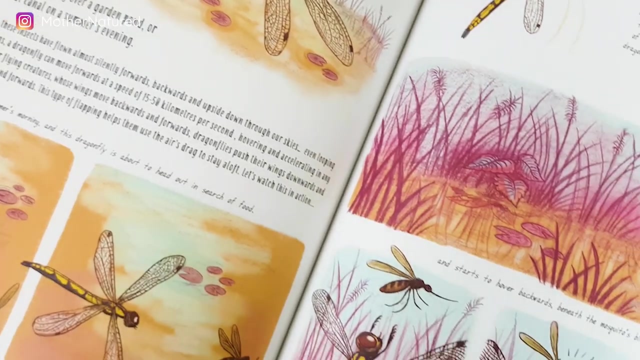 because they're all collaged So they almost, you know, pop off the page in 3D We just bought. this is a brand new book that we've just bought and I love it already. It's called Slow Down and it's got just different moments in nature that have a story to it, So I'll 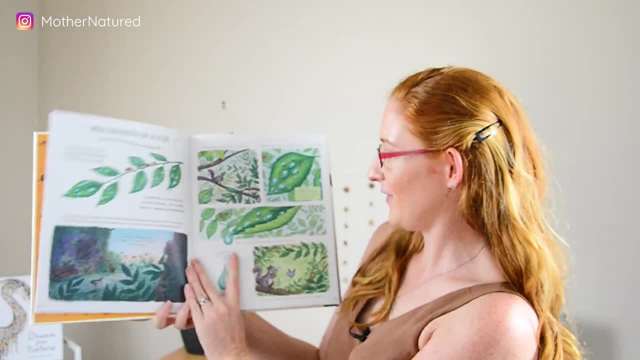 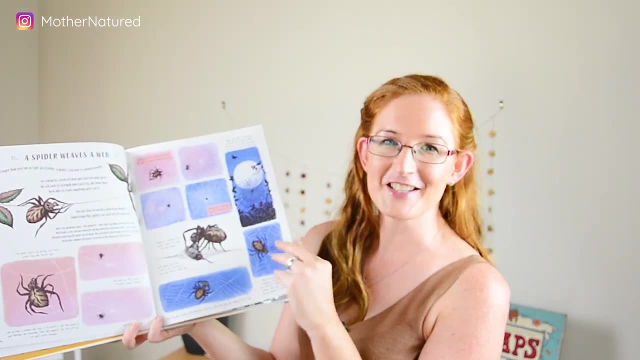 give you a quick example. but you know, dew collects on a leaf, So something so simple. but there's a story surrounding that. A spider weaves a web and, as you can see, the illustrations are really sweet: A thunderstorm on a sunny day, So it's really taking snippets of nature. 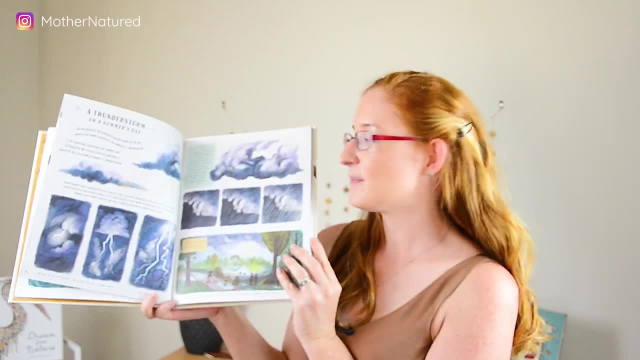 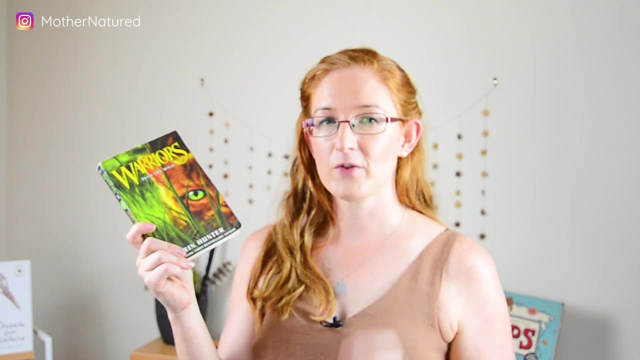 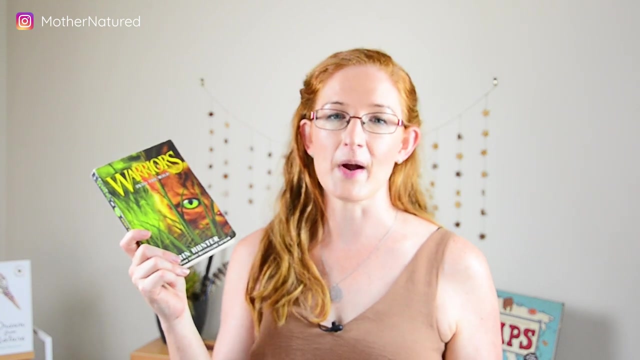 and forming a story around them, and it would just be beautiful to share with children on. you know, at night before bedtime, The eldest daughter is really into warriors. She gets fully immersed in it. These cats are wild and they live wildly and they interact wildly, and so she feels like she's taken away into this other world where she is a cat in nature. 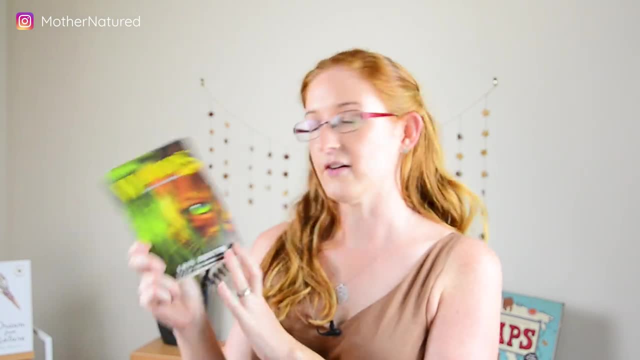 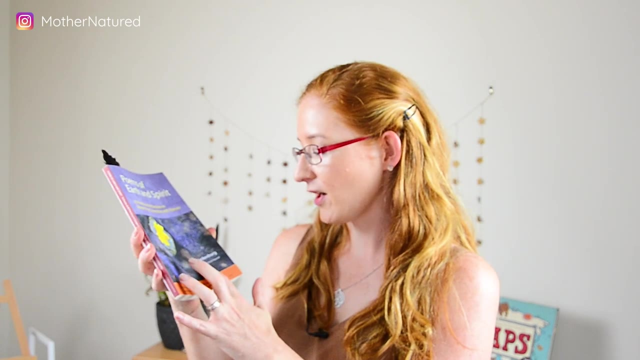 So she's addicted to this series- Warriors by Erin Hunter. Another book that I really wanted to show you- that wasn't really a picture book sorts, it was Poems About Earth and Spirit by Kai Sedenberg. I hope I'm saying that right, But it's. 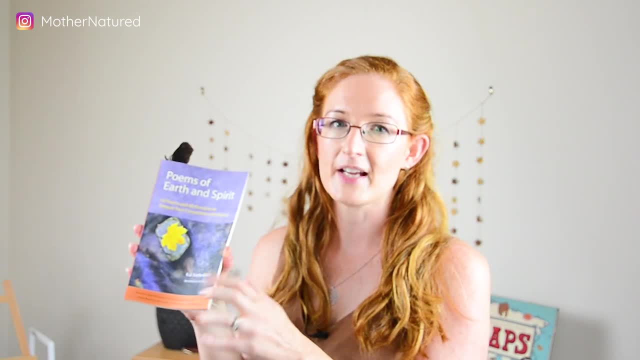 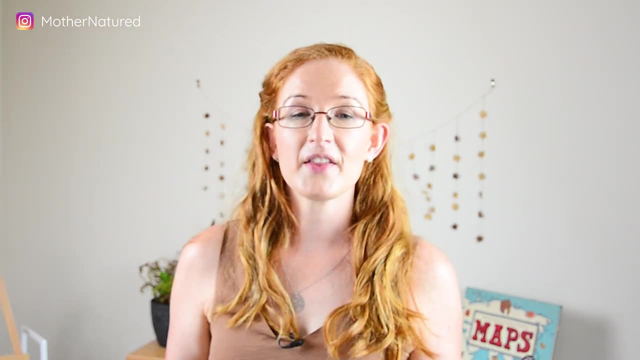 70 poems and 40 practices to deepen your connection with nature. And this book is filled with lots of beautiful ones, some that have little stories, some that just really help you to reflect, And I think reflecting is a really good thing that we can be doing with our children right now, or just even. 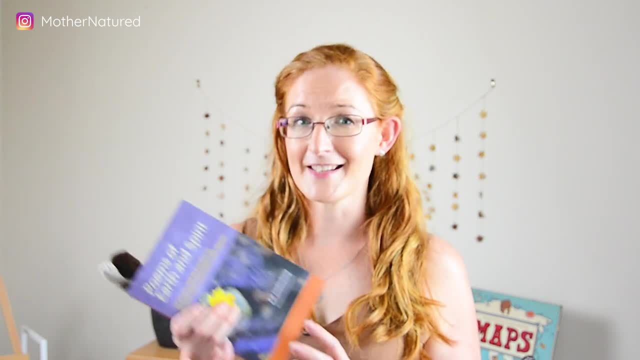 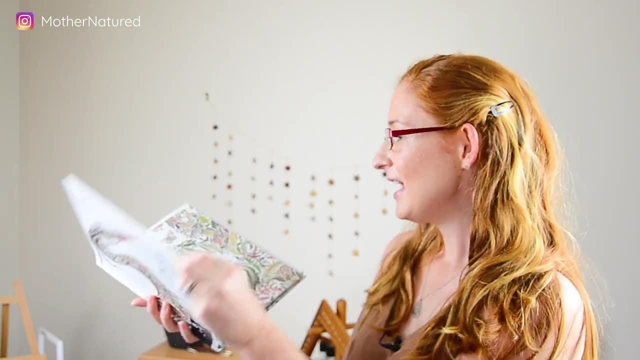 you if you feel like poems are something that might resonate with you. This is quite a sweet book. Oh, I forgot one more book that I really love, that we recently bought too. It's Drawn From Nature. It's very up my alley because I love nature crafts, because all of these illustrations 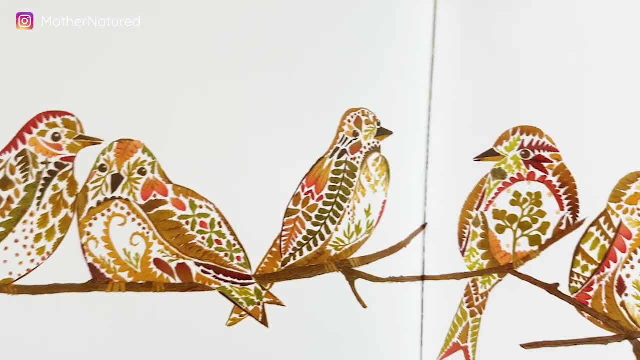 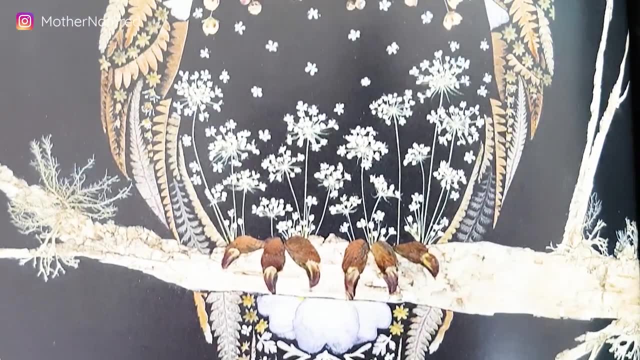 I haven't had a chance to fully read it yet, but the illustrations just captivate me So I'm sure I'm going to love it either way. But they're all the silhouette. the whole animal is made out of nature And it's just incredible We don't tend to buy a lot of nature books. 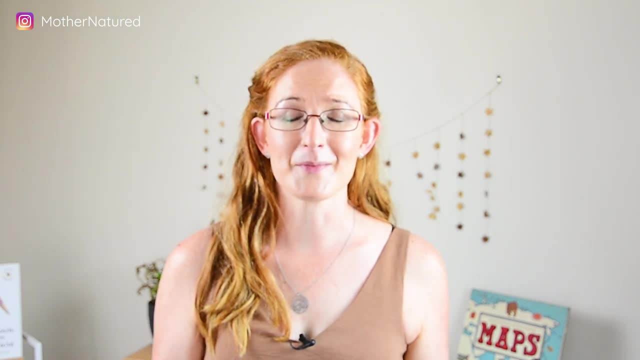 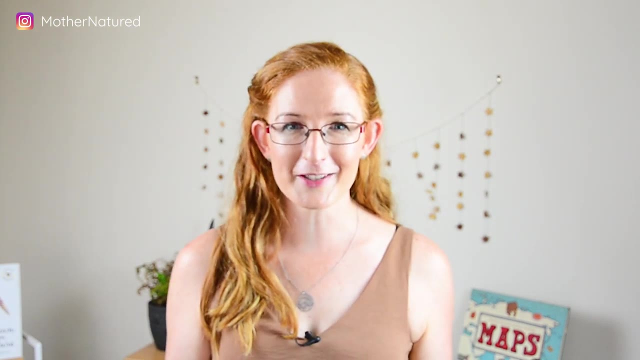 we borrow a lot of books, But our library is at the moment closed So we can't go there. Oh, I miss the library. Is your library closed? Let me know. in the comments below. I'll add a link to all the books that I mentioned. 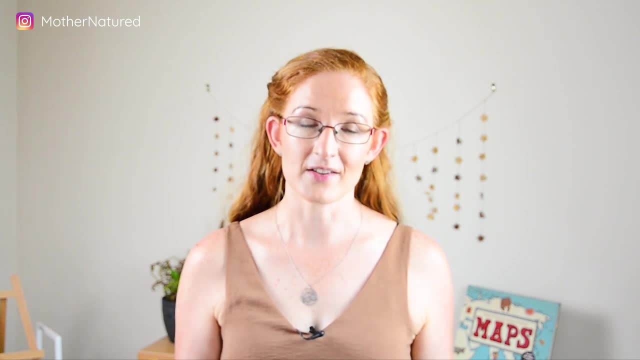 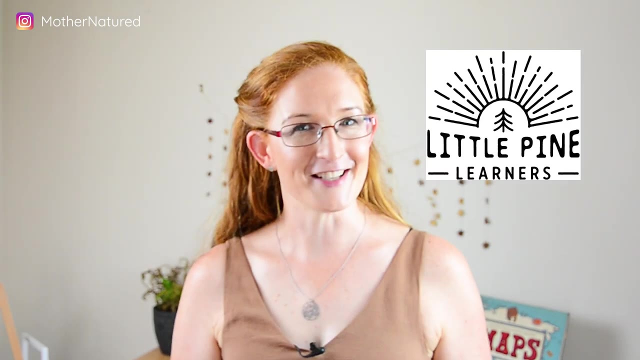 in the description below. But just so you know, they are affiliate links, So that means that if you click on the link and you buy it, I do get a small commission at no cost to you. My friend Tara from Little Pine Learners has this wonderful idea called Window Nature Prompts. She suggests that you 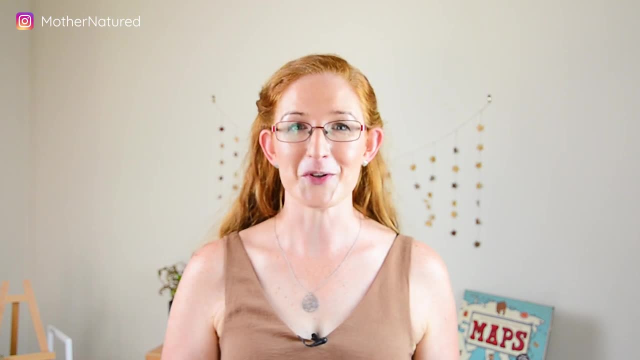 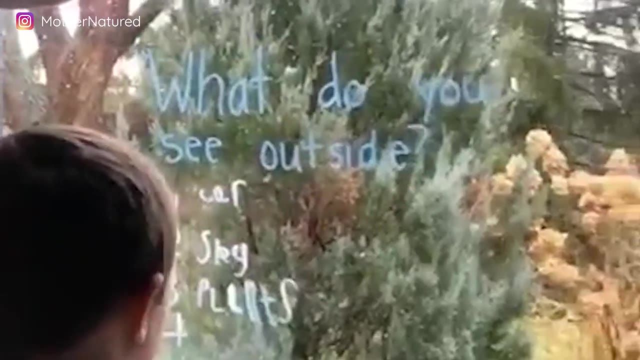 write or draw pictures on your window with a dry erase marker or a liquid chalk marker. Now they're easy to come off, just with a damp towel cloth. You can draw a scavenger hunt up on the window And each time your child sees something through the window they have to tick it off, Or you can get.